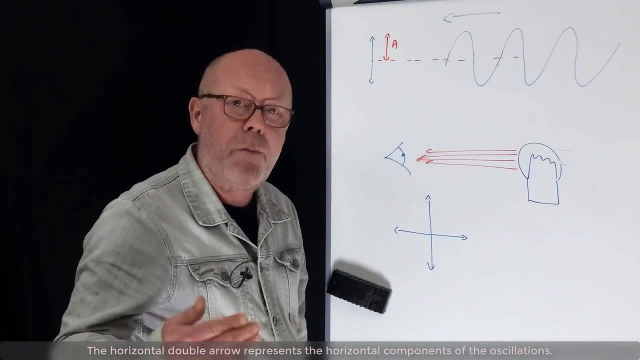 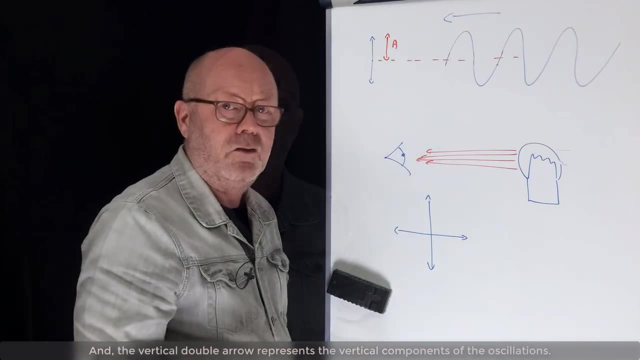 The horizontal double arrow represents the horizontal components of the oscillations and the vertical double arrow represents the vertical components of the oscillations. In order to transform unpolarized light into polarized light. in order to transform unpolarized light into polarized light. 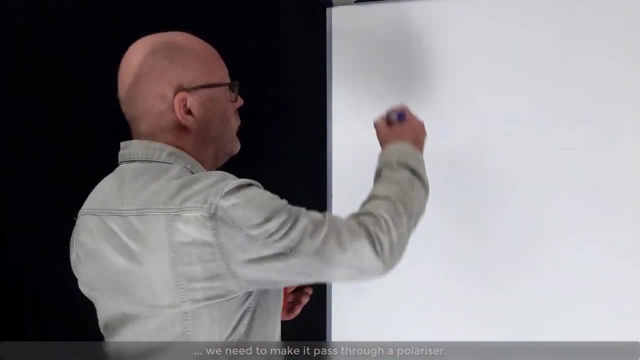 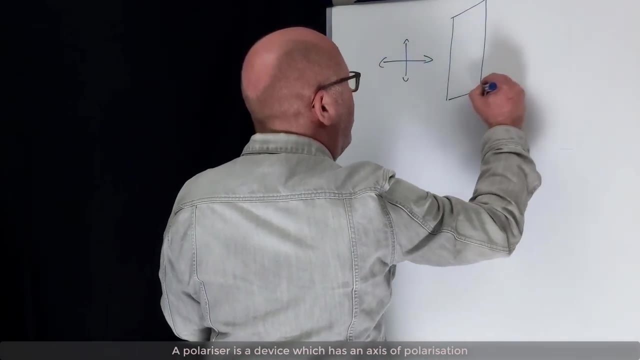 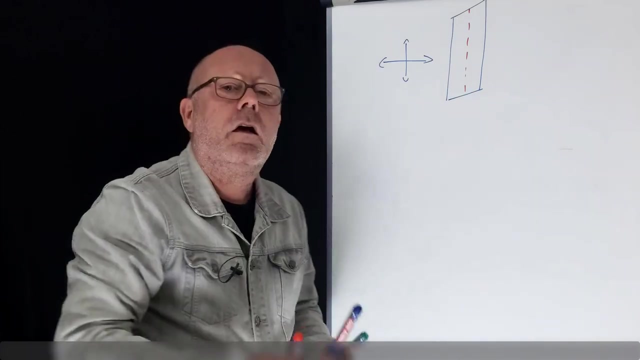 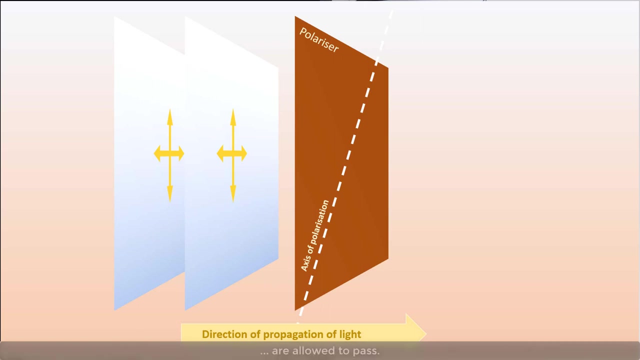 we need to make it pass through a polarizer. A polarizer is a device which has an axis of polarization. Here I choose it vertical. Only the components of the light which are parallel to the axis of polarization are allowed to pass. So what comes out of the polarizer is light oscillating. 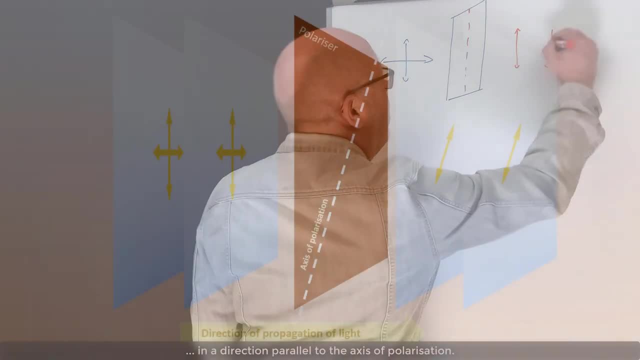 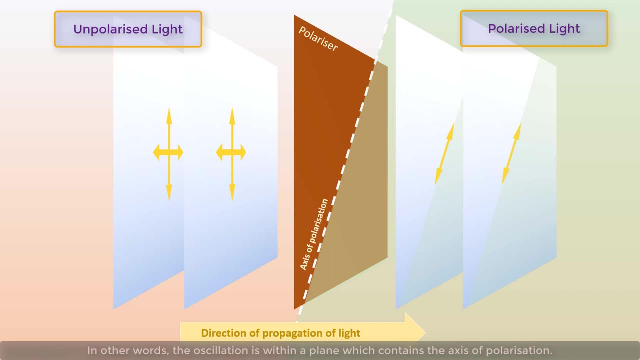 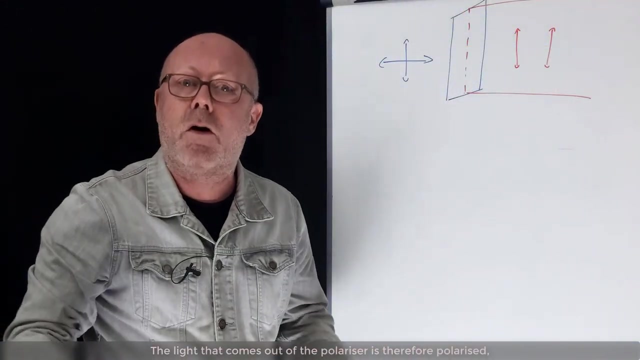 Is light oscillating in a direction which is parallel to the axis of polarization. In other words, the oscillation is within a plane which contains the axis of polarization. The light that comes out of the polarizer is therefore polarized because it's oscillating in one plane only. 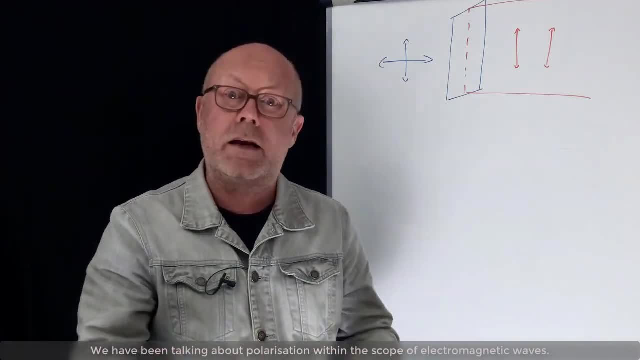 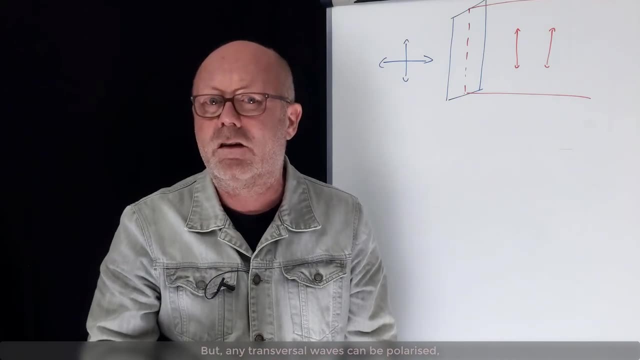 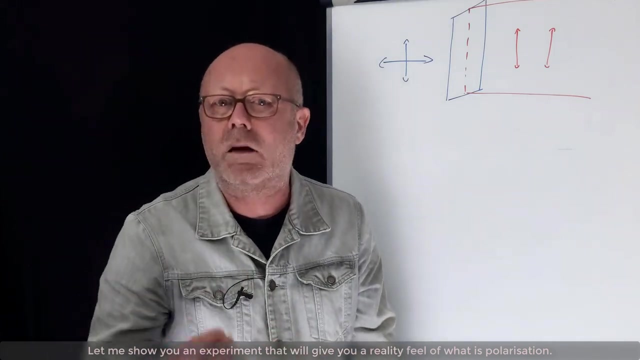 We have been talking about polarization. within the scope of electromagnetic waves, Light, basically- Any transversal wave can be polarized, even mechanical ones. Let me show you an experiment that will give you a reality feel of what is polarization. This is my oven rack. 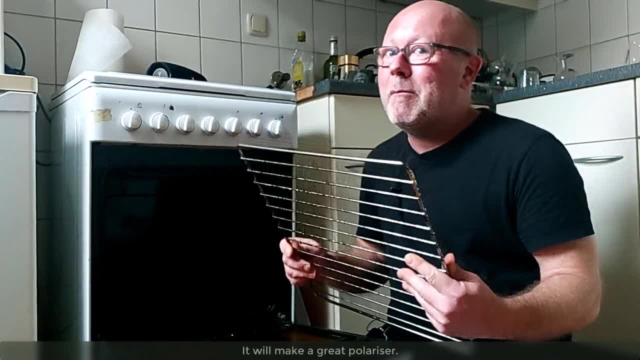 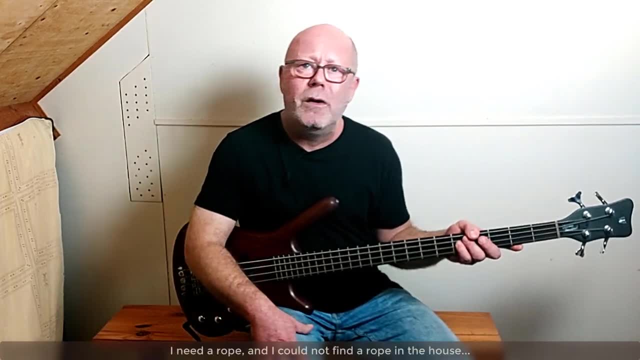 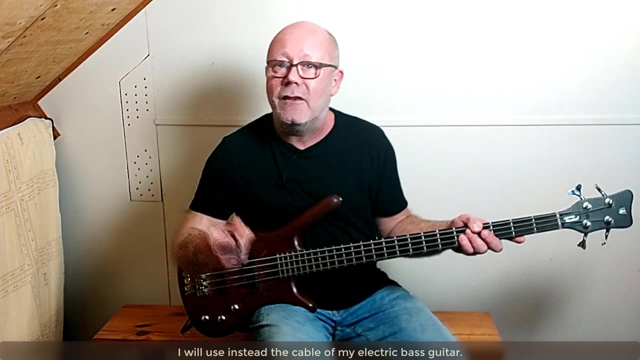 It is made of parallel metallic bars and it will make a great polarizer. I need a rope and I couldn't find a rope in the house. Yes, I need a rope to show you something, So I will use instead the cable of my electric bass guitar. 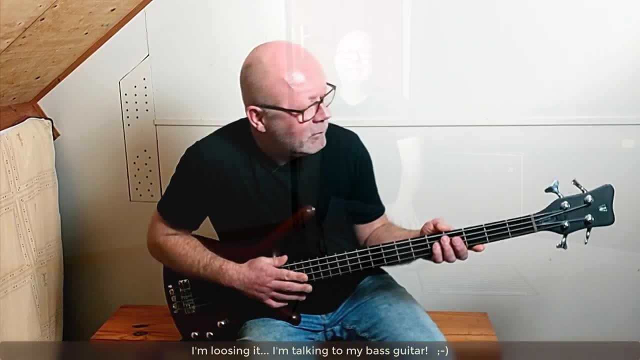 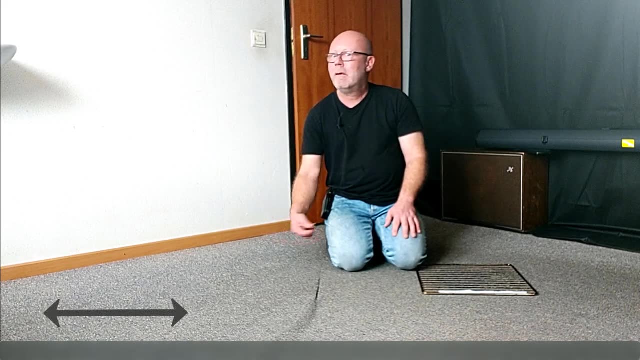 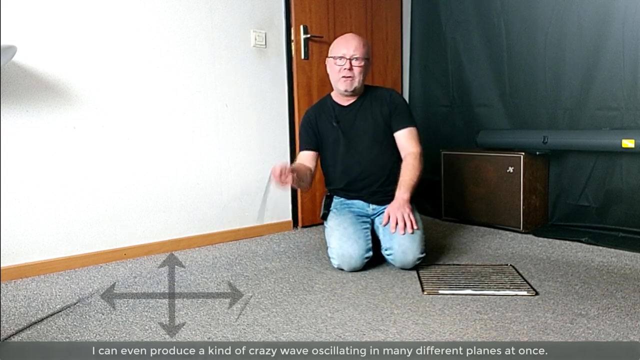 I hope you don't mind, baby, It's for a physics experiment. By shaking the cable I can create a wave oscillating in the horizontal plane Or a wave oscillating in the vertical plane. I can even produce a kind of crazy wave oscillating in many different planes at once. 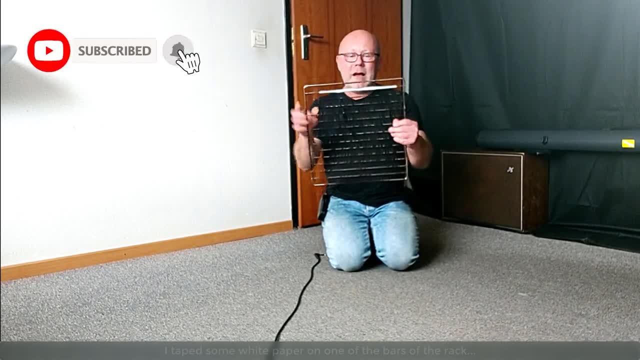 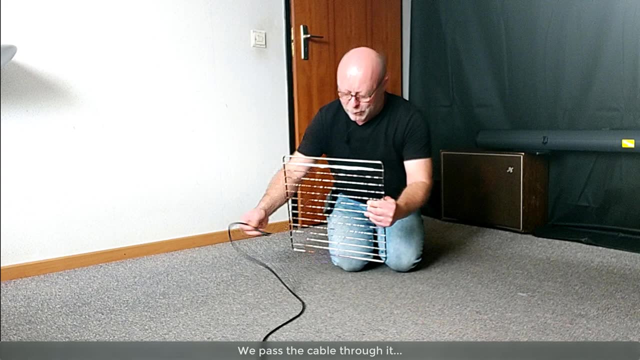 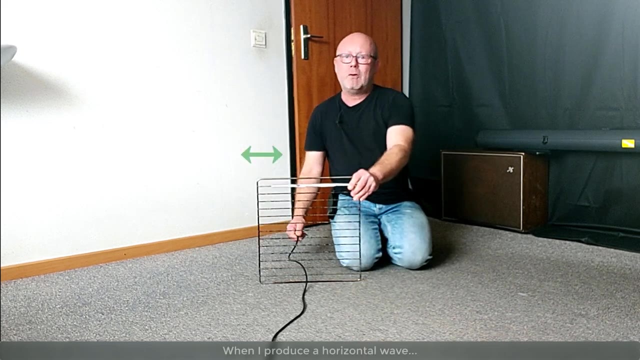 This is our improvised polarizer. I taped some white paper on one of the bars of the rack so that you can see the axis of polarization. I will pass a cable through it and set the axis of polarization horizontal. When I produce a horizontal wave, it's like if there was no polarizer. 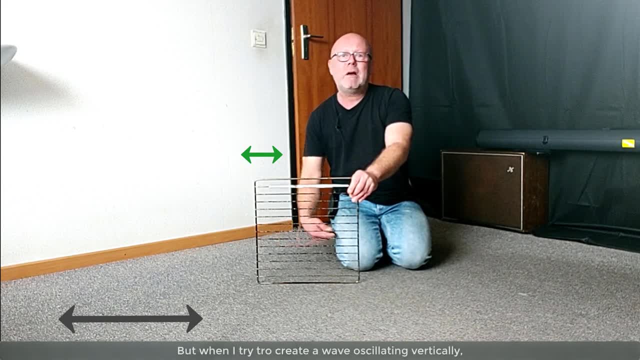 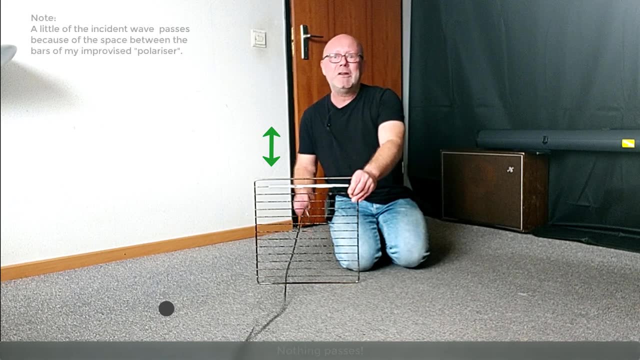 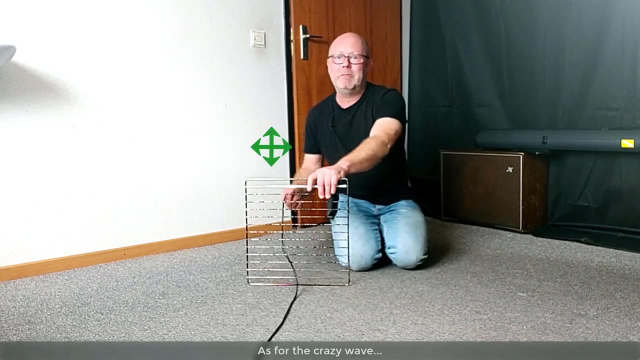 The wave passes fully, But when I try to create a wave oscillating vertically, nothing passes. Yes, the vertical wave has no horizontal component, so it is fully blocked. As for the crazy wave, Difficult too, As you can see, only the horizontal component passes. 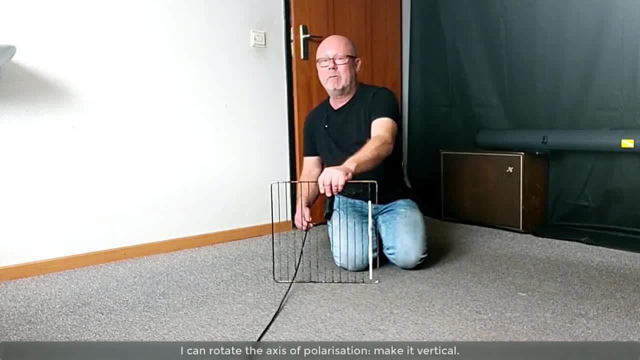 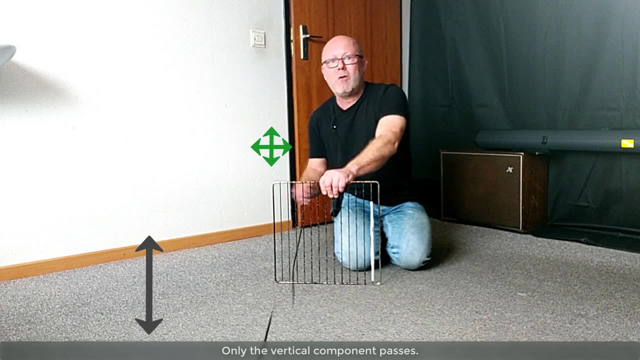 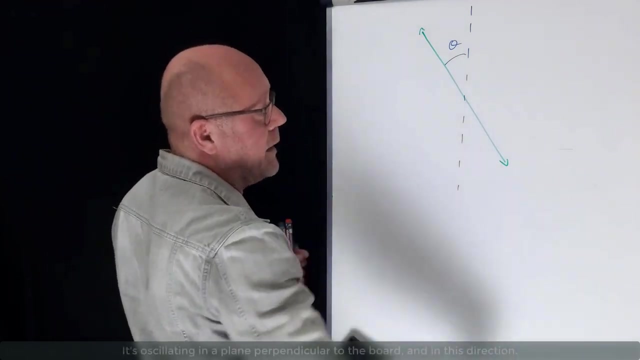 I can rotate the axis of polarization, Make it vertical. Now it is the horizontal component which is blocked. Only the vertical component passes. The green double arrow here represents a wave coming towards you. It's oscillating in a plane perpendicular to the board and in this direction. 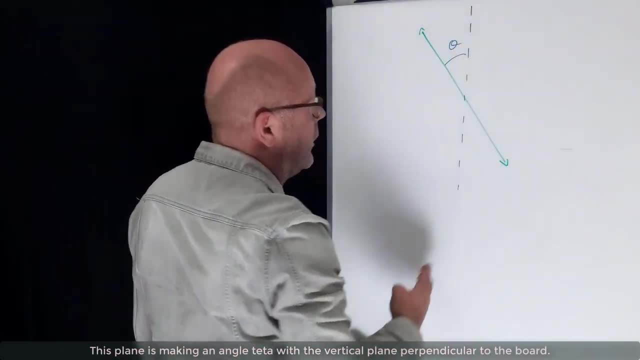 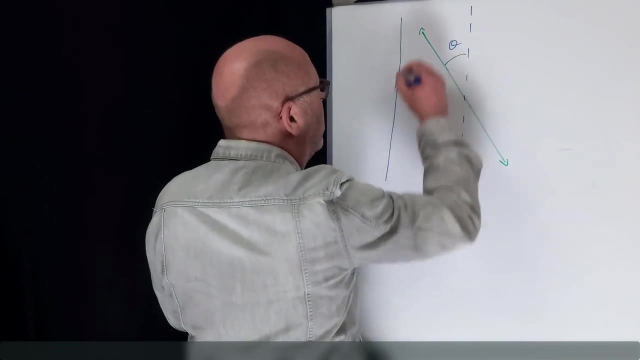 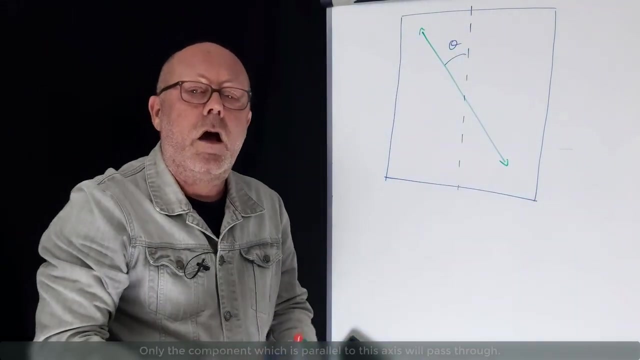 This plane is making an angle, theta, with a vertical plane perpendicular to the board. Imagine now that I place a polarizer between you and the wave And I will choose the axis of polarization of this polarizer being vertical. Only the component which is parallel to this axis would pass through. 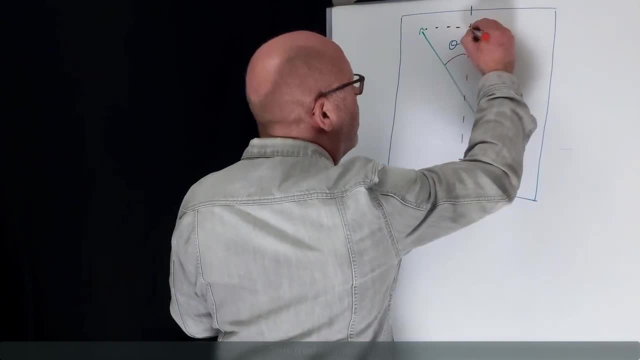 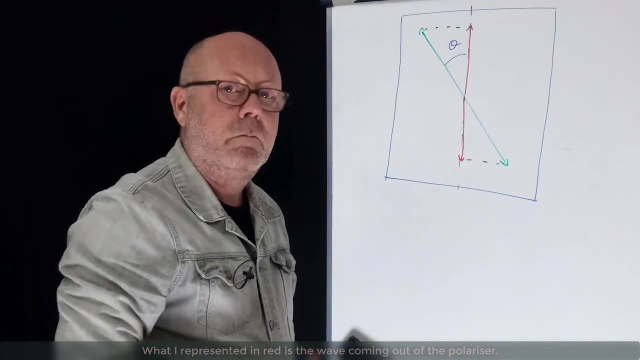 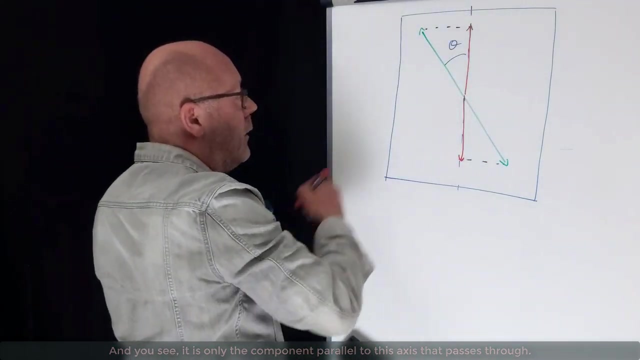 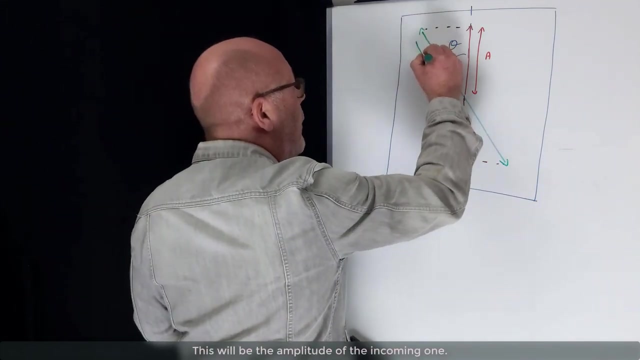 That is this. What I represent in red here is the wave coming out of the polarizer, And you see that it's only the component parallel to this axis that passes through. This will be the amplitude of the output wave. This will be the amplitude of the incoming wave. 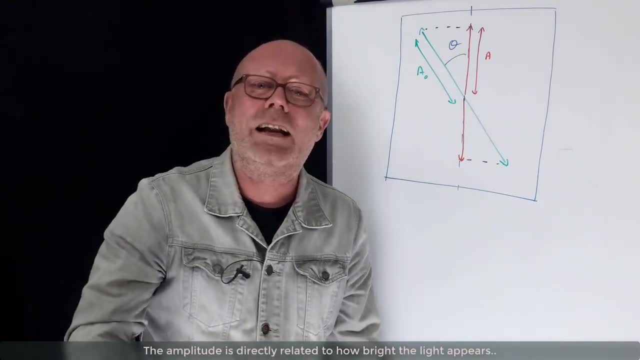 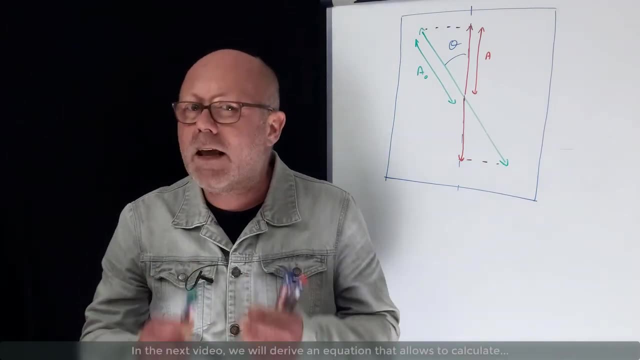 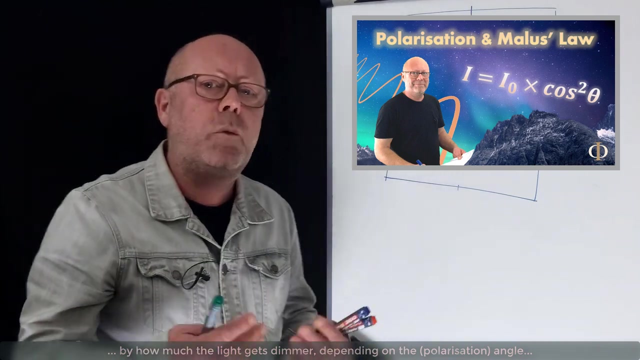 You see that the amplitude decreased. The amplitude is directly related to how bright the light appears. So passing through a polarizer dims the light. In the next video we will derive an equation that allows you to calculate by how much the light gets dimmer, depending on the angle at which the light comes in the polarizer. 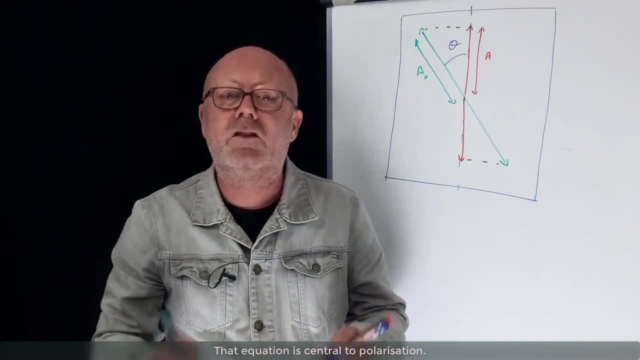 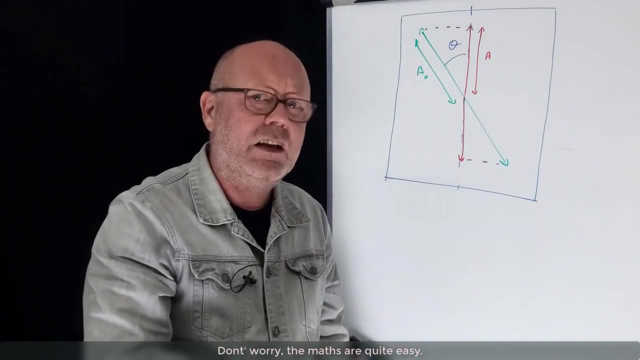 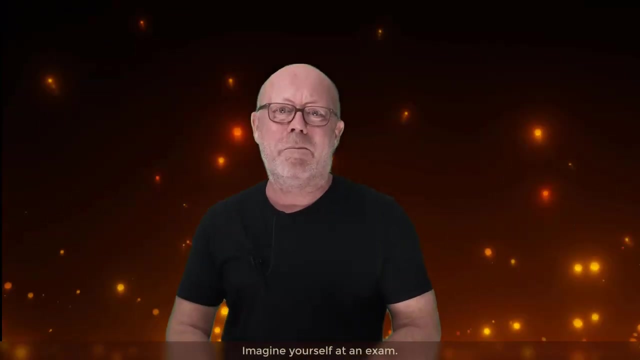 This one, the angle theta. That equation is central to polarization. It is called Malus law. Don't worry, The math are quite easy And it will be a cool video also, So stay tuned. Imagine yourself at an exam. You are reading the questions.